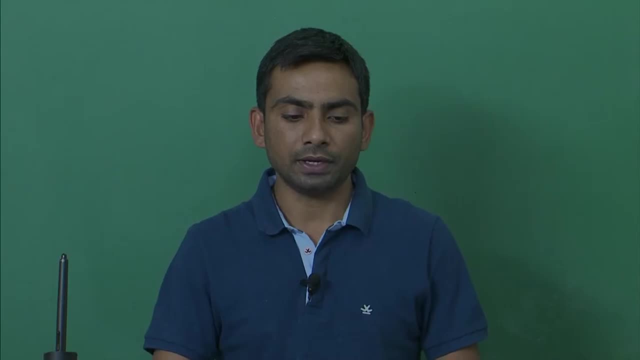 and in the present module 26 and 27,, I will discuss a new topic called material selection in engineering design. This topic is very important topic for the design purpose. For example, if you want to convert your idea into your practical product, then what you 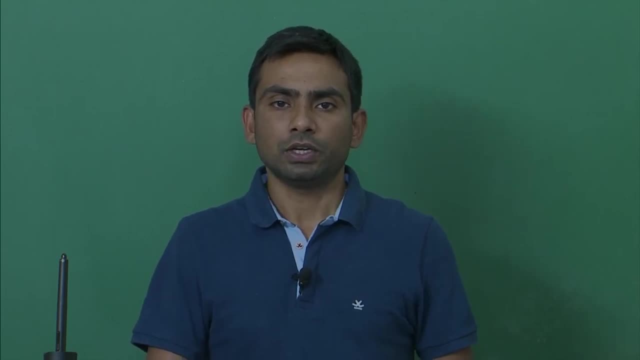 will do. You will require a material to fabricate it. So you know that in universe we have a variety of materials available. So to choose appropriate material for your particular product there are some processes needed. So in this module you will learn these things. 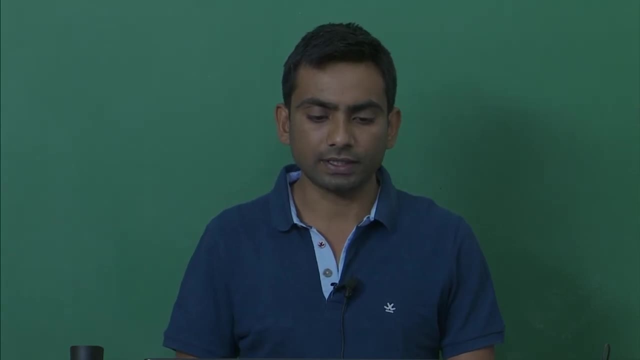 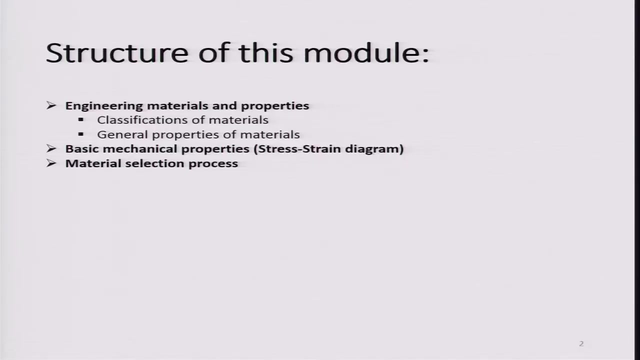 So in that this kind of things we will discuss in our coming module, And structure of this module is following: First we will study some engineering materials and properties, then their classification of some materials, Then again generalization of some materials, Then 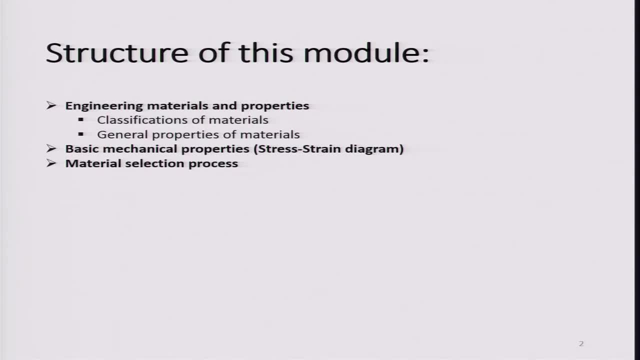 again generalization of materials, Then again generalization of some materials, Then again material properties of materials. then, since in this module we will focus only on mechanical aspect of designing, So we will study some in brief mechanical properties, such as, for example, stress-strain diagram and etcetera, And after that we will study material selection. 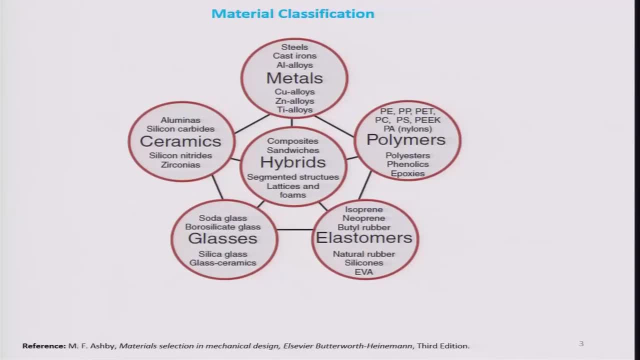 process. Now material classification. in this we know that there are variety of materials available in our universe and these are broadly classified in these groups: metals, polymers, ceramics, glasses, elastomers, hybrids. Metals are generally in crystalline in nature. 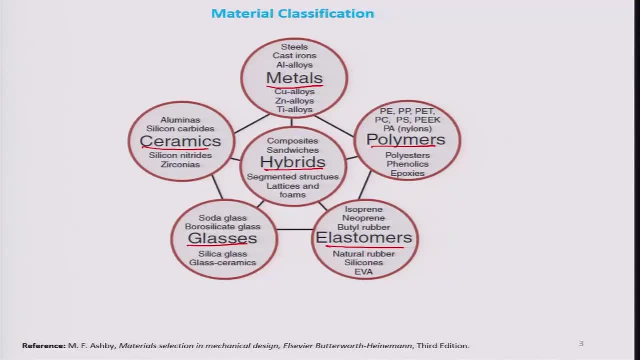 and the atoms of the metals are held together by metallic bonding. These metals are very strong and hard and some materials are ductile. some materials are very brittle in nature and we will study these things in detail in coming in next slide. Now ceramics. ceramics are also. it may be crystalline or non-crystalline. 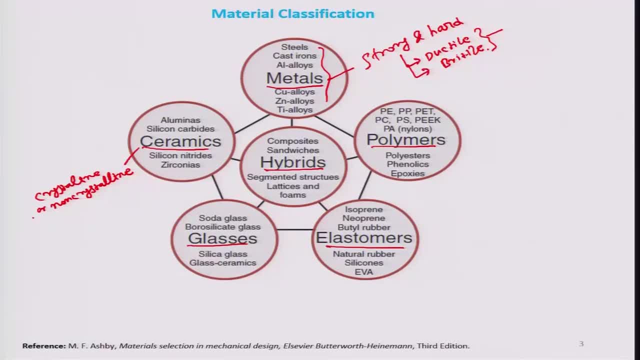 and here molecules are bonded with ionic or the covalent bond. ceramics are very higher strength, possesses very higher strength, while in compression ceramics are generally brittle in nature. So when you will apply a tension in this metal, So there will be a. it will fracture immediately. in comparison to metal, a fracture. 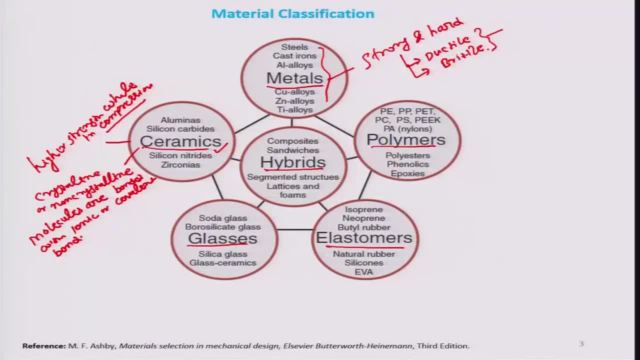 will take place in a very earlier time. So, and this also- these materials are electrically insulate, chemical inert, etcetera, Polymers, polymers it is. it is made with many repeating mers to form very large molecule And molecules are bonded with covalent bonding molecules and several elements are present. 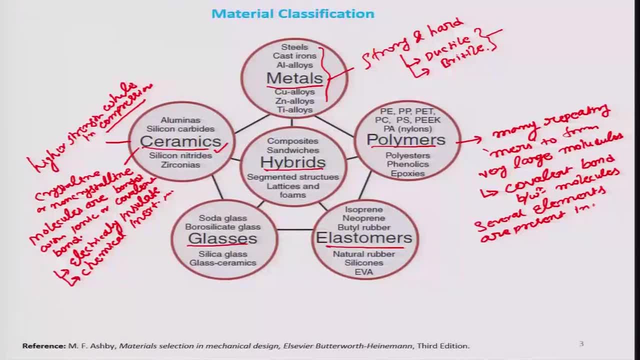 in polymers, In ago, the elastomers. you can take examples of rubber for met metals. we have a variety of metals available in our universe, such as aluminum, iron, bronze, etcetera. 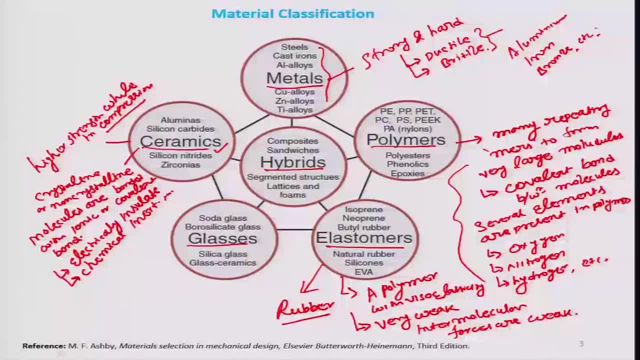 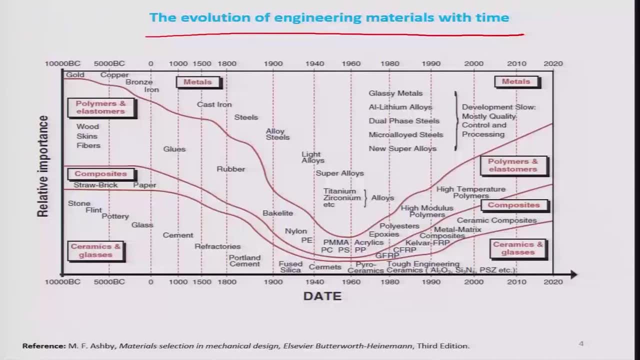 that variety of materials- gold, copper, bronze, iron- and their advent time is mentioned here, So in stone age, that is, the 10000 BC, and here some materials were discovered that was 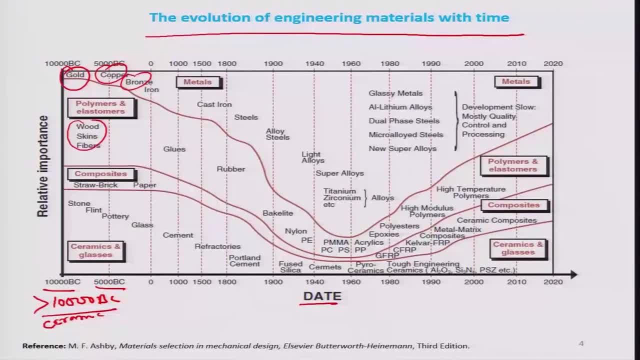 the ceramic, wood, skin fibers, woods and stone were used as a for their armory and in a bronze age bronze area that is the time period between 4000 to 1000 BC, Here bronze were developed, discovered in iron age. iron age lies between 1000 to 1620. 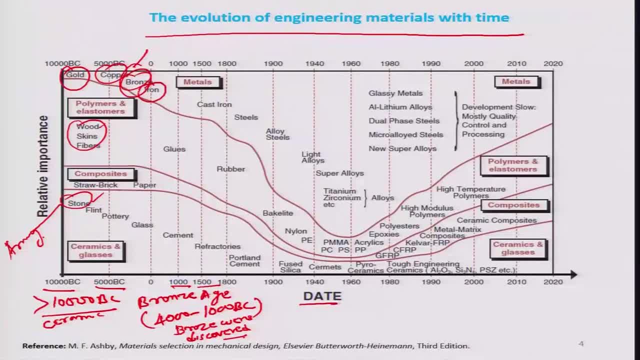 BC, and here you can say irons, cast iron and some natural glue from the tree was discovered. So here bronze was discovered And in cast iron was first was dominant in 1620s. and we, but you can see from this plot, 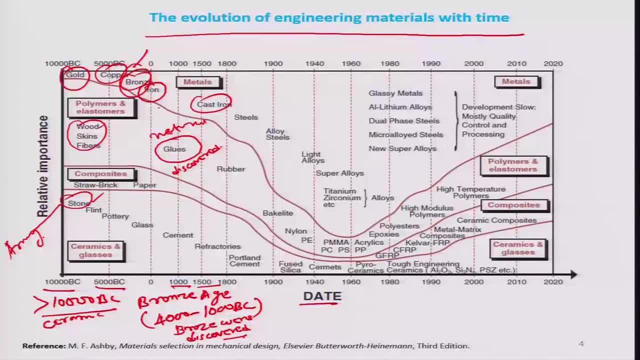 that the these materials, the use of these materials, continuously decreased with the time and as well as their new materials, was discovered at span on a time span on time. We can see that in 1850s steel was discovered. steel, It is another form of iron, purified form. you can say. 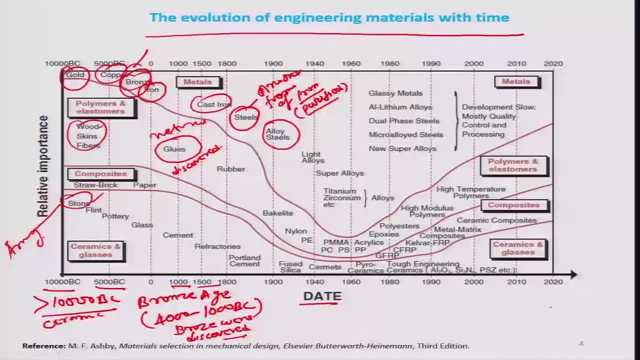 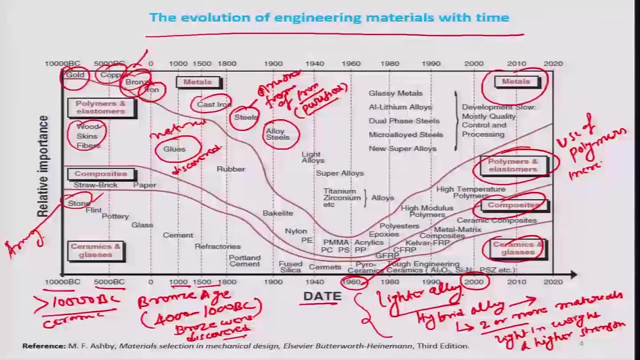 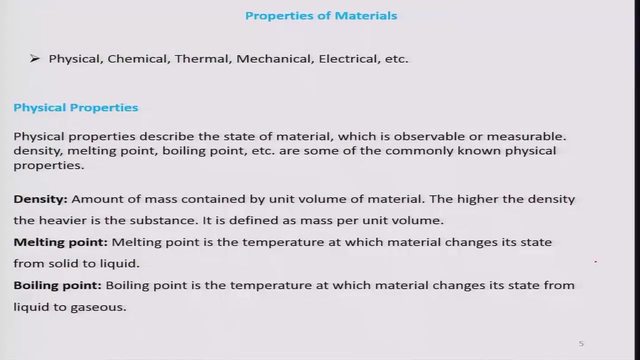 Now, after that, from the 1940s, 60s, now people approaches towards the light alloy, lighter alloy, And amount of the mass content by unit volume of the material. if any material has a, suppose that iron has a higher density than aluminum. 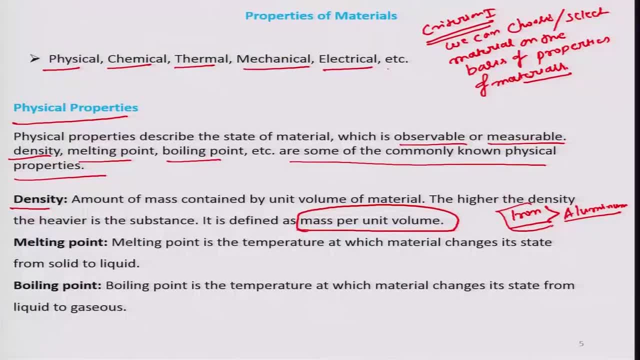 It means if you fabricate something using iron, that weight will be…. Times Is Aluminums credible, So suppose that if you take a constraint, that material massive part should be lighter. 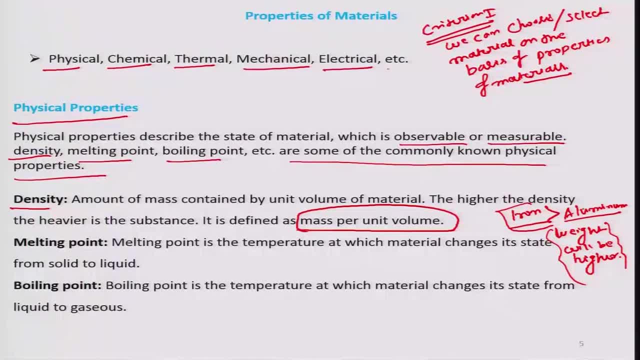 in weight. So you will have to choose very intelligently which material will be suitable for your product. Melting point: melting point is the temperature at which the material changes its state from solid to liquid. For example, iron has a melting point of about 15-30 degree. 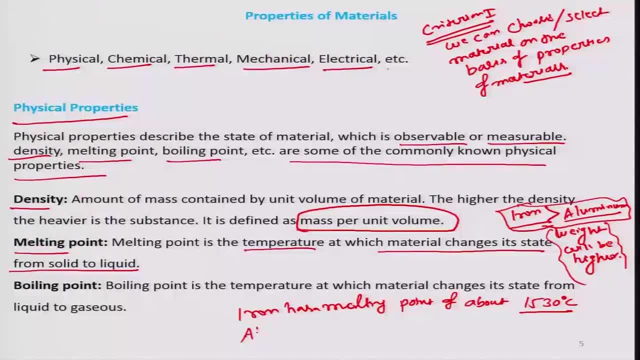 Celsius, While aluminum has a melting point of about 15-30 degree Celsius. So this is the melting point around 660 degree Celsius. So you can see that at 660 degree Celsius, aluminum will get melt, melted away at 6 degree Celsius, While at 660 degree Celsius, iron. 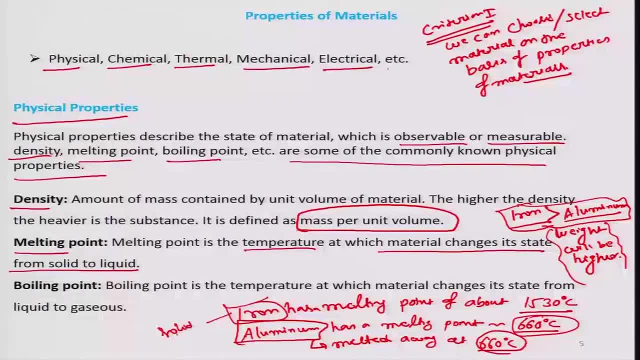 will be present in solid form. Boiling point: boiling point is the temperature at which the material changes its states from liquid to gaseous. So boiling point, you know, everybody knows that boiling point of water that is the 100 degree Celsius. It means at 100 degree Celsius liquid will start boiling. 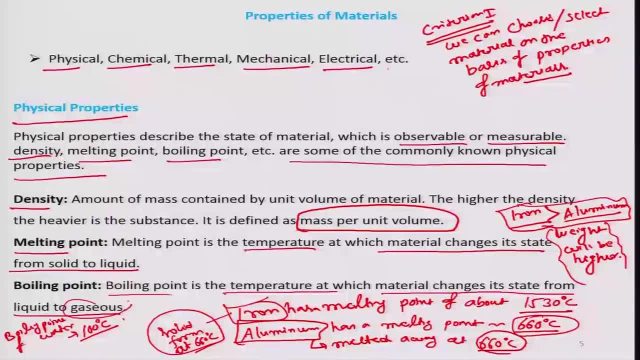 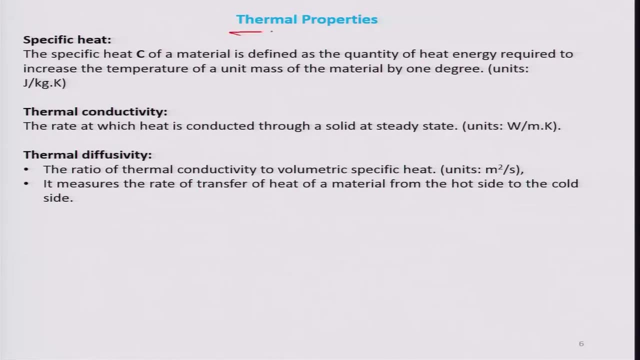 be, it will start converting into gaseous media. These are the main permanent physical property of any material: density, melting point, boiling point, etcetera. Now we will talk about thermal property. Every, each material has thermal property. What is the thermal property? It is a thermal property means transfer. 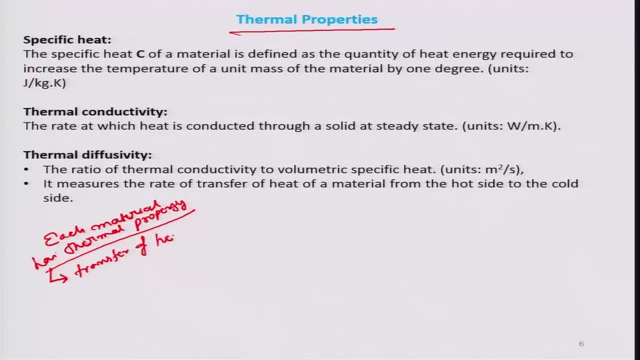 of heat through media. that is the conduction It can be, and heat transfer can take place using conduction convection. 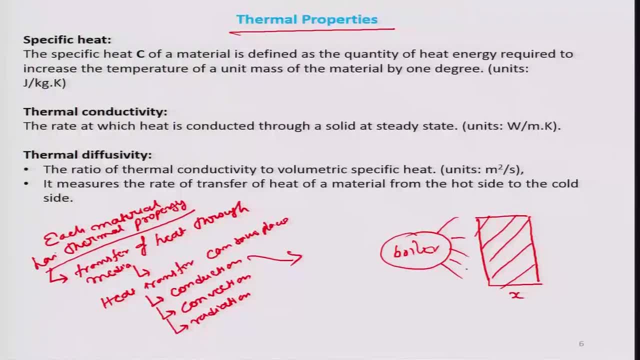 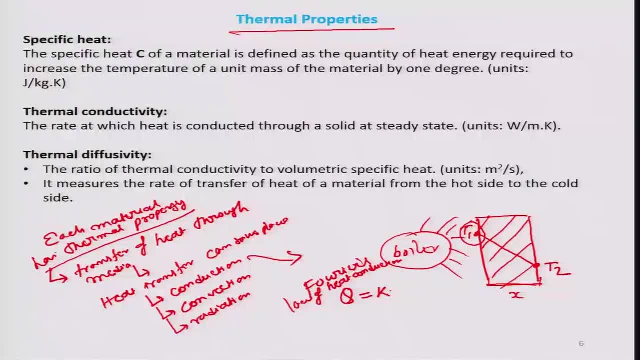 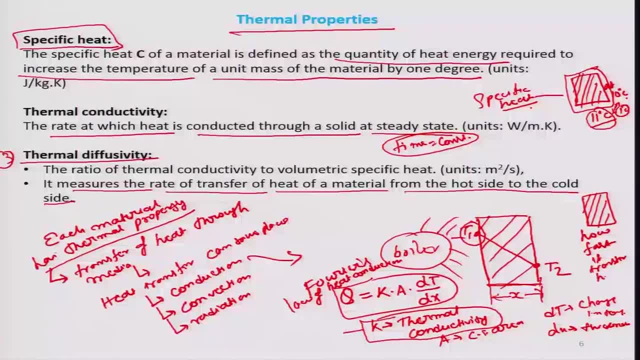 And it can be calculated as thermal diffusivity signifies as alpha. alpha is equal to k by rho- c, where k is the thermal conductivity and c is your specific heat of material and rho is the density of the material. So if you know density of material, specific heat. 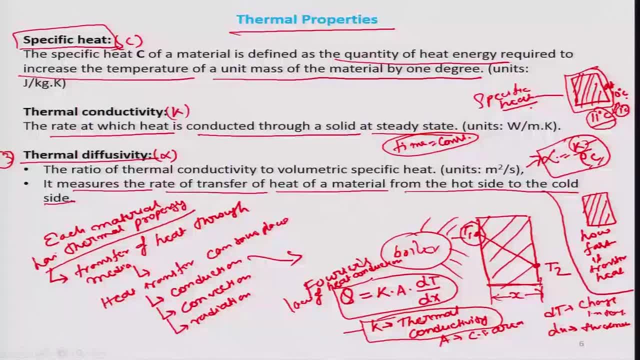 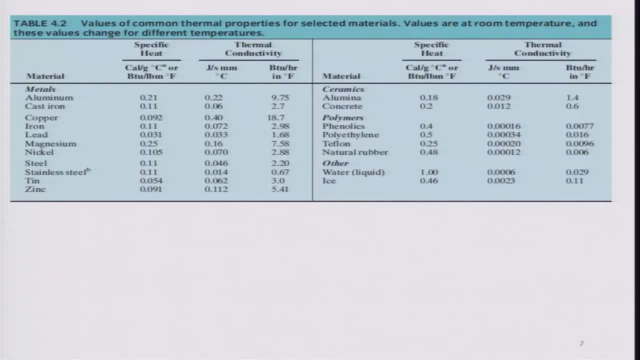 and thermal conductivity, then you can easily calculate the thermal diffusivity of that particular material. This table shows the way some common thermal properties of selected materials and you can see: for metal, such like, for example, aluminum, the specific heat is 0.21, for cast iron it is 0.11, copper 0.092,, kerosene it is 0.2,. 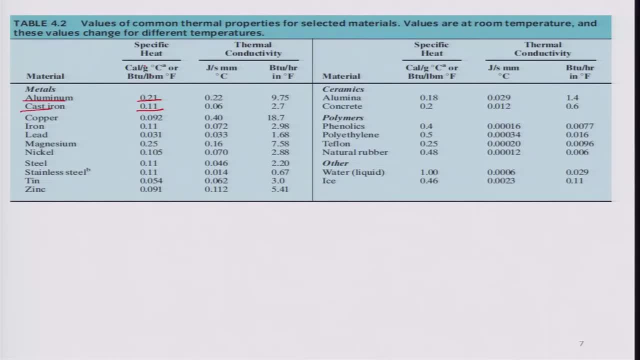 kilo kelvin. kelvin per gram into kelvin Thermal conductivity, if you see, the aluminum is 0.22 joule per second mm. for cast iron 0.06, for zinc 0.112.. So in comparison what? 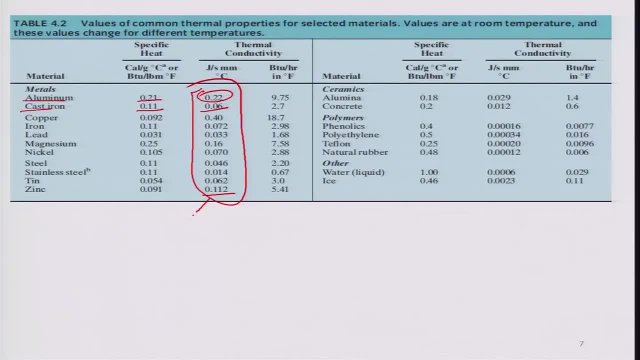 you are getting aluminum. thermal conductivity of aluminum is higher than thermal conductivity of copper. So for cast iron also, thermal conductivity of copper is higher than these two. So it means we will conduct heat at faster rate As compared to aluminum and cast iron. some another ceramic, you can say alumina, 0.029,. 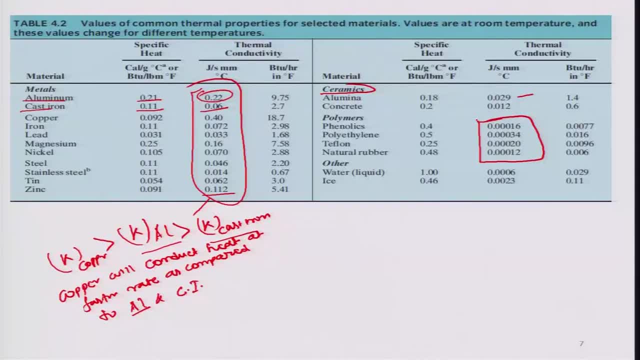 polymers are very poor in heat conducting. these are the very Now some other properties of material. is that optical property an optical property? it depends on wavelength and types of material. another parameter which can affect the optical property is the incidence angle. suppose that here is your one material and 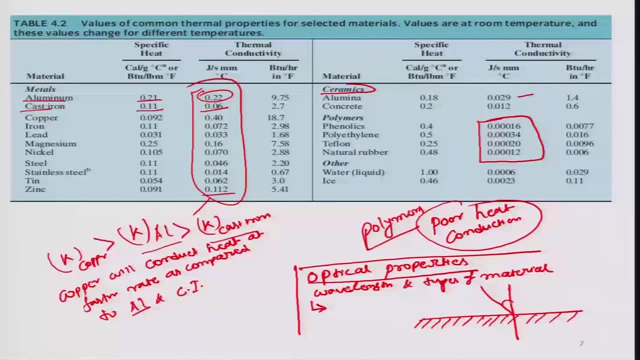 light is coming like this: that is the theta I, it is the angle of incidence that is make through the perpendicular to the, your material and its get reflected. that is the reflection and that is the transmission incidence. okay, so algebraically, in soul, incident intensity, I, I plus I, R plus I, T will be one. 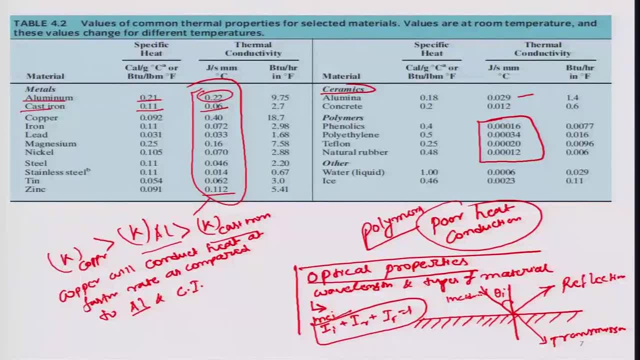 some materials are very reflective in nature. some materials are transfer time, very poor reflection position, very poor reflection. so these properties are important if you want to design- suppose that microscope, for example, micro scopic lens. So these optical property will play predominant role, but in this module we will focus only 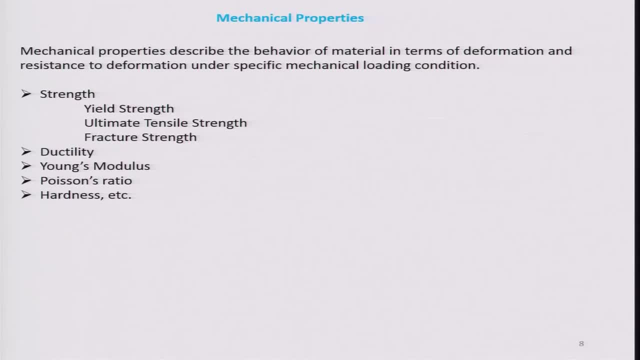 on our mechanical part, mechanical properties, So mechanical property. this describes the behavior of material in terms of deformation and resistance to deformation under specific mechanical loading condition and they are the various properties of comes under a mechanical property. that is, a strength, yield strength, ultimate strength of the material. So we 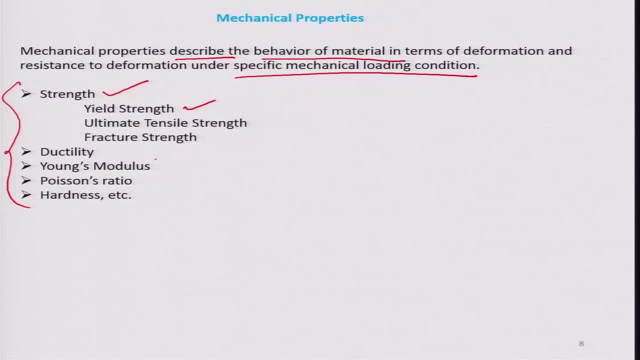 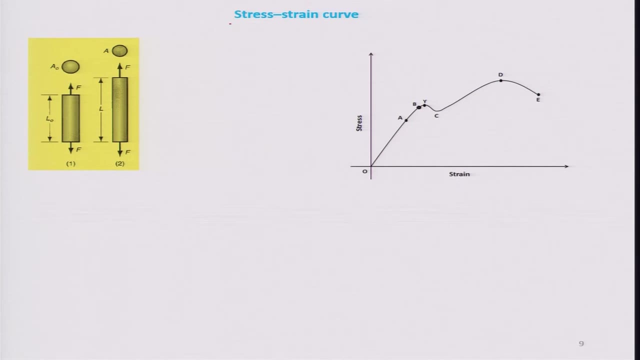 will talk about the potential strength fracture: strength, ductility, Young's modulus, Poisson ratio, hardness. we will study in detail in these things in coming slide. first we will start from the stress strength diagram here. what we are doing, we have. we take one bar. 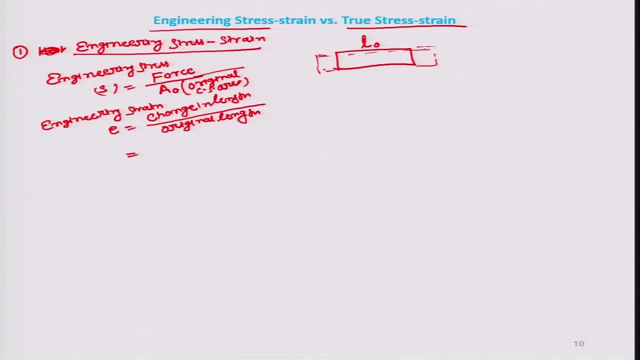 applied load length for particular at a particular load length is L, So change in length will be L naught minus L naught divided by L naught, this is the L naught minus L naught. So this is L naught minus 1, where L is equal to length at any point during the elongation. So Hooke's. 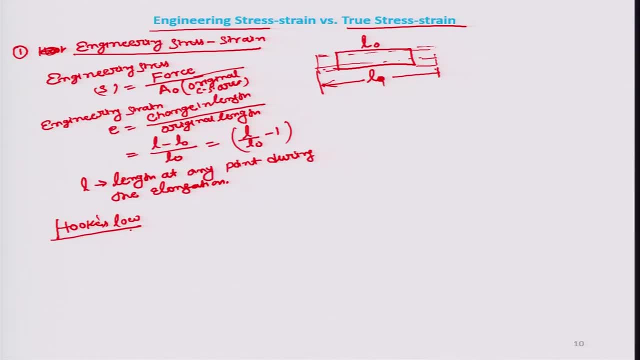 law of linearity for up to the power for point. So O, A, what will be happen? Stress is directly proportional to strain and E to E, where E is the modulus of elasticity. So it is a measure of the inherent stiffness of material. So 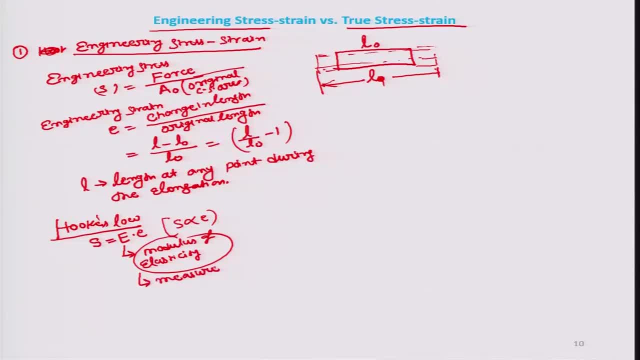 it is a measure of the inherent strength. Now we will study proof of stress strain. ok, What is the true stress? It is the ratio of force per unit area. that is the actual area means for a particular load. F length is increased to L and cross sectional area is changed to. 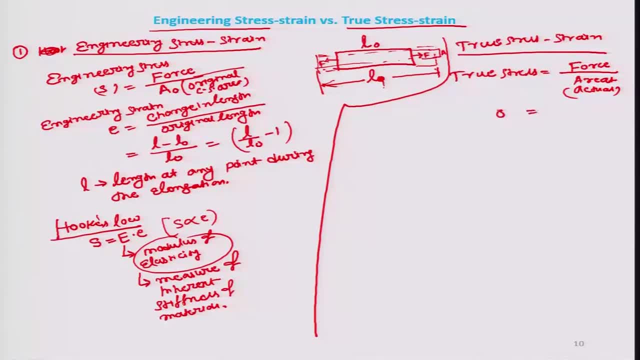 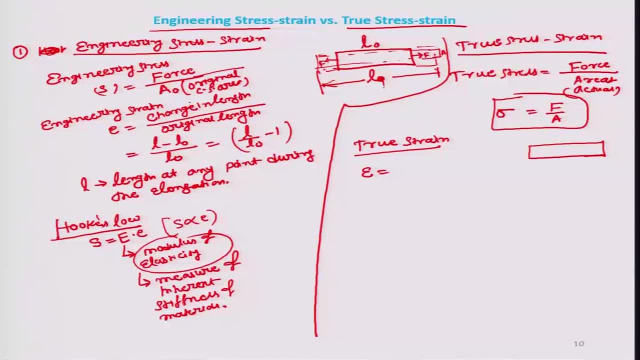 of load. So we can write that using same thing: change in length divided by original length. So suppose that first initial length was L naught and final length is L. So we can write that using same thing: change in length divided by at particular load and change. 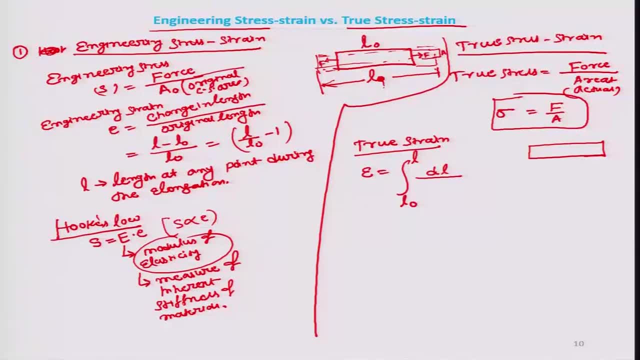 in length. what is D, L and initial? And if you will solve log L by L naught? So if we substitute the value of L naught from here, so what will happen? So that is the initial length and change in length. what is D, L and initial? and if you? 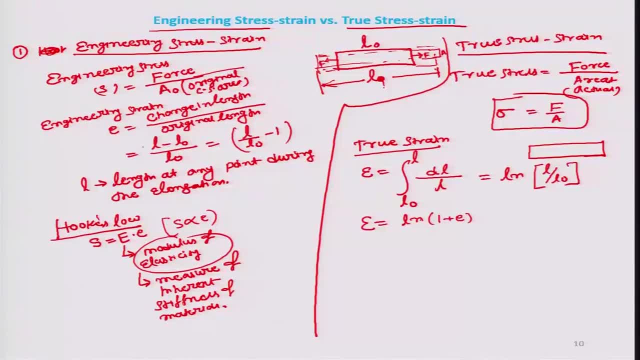 1 plus E. This is the relation between true strain versus, and engineering strain means 2 strain is equal to l n 1 plus engineering strain. Similarly, we can derive an expression for true stress versus: 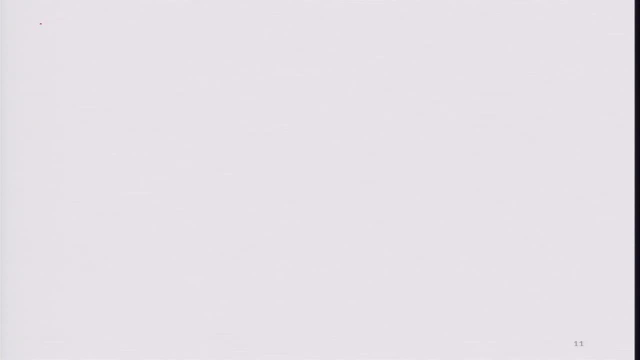 deformed without failure. And if you want to quantify ductility, then you will have to measure either percentage elongation or area reduction. 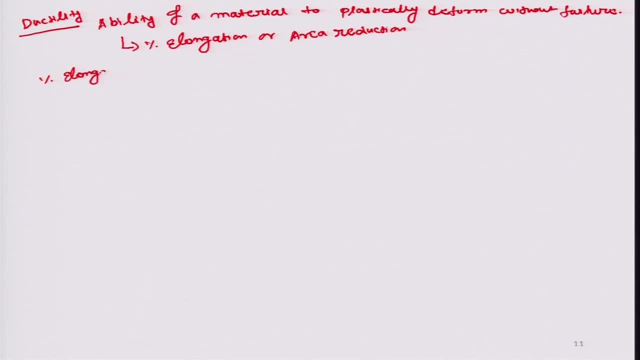 What is the percentage elongation? It is the ratio of difference between final length and final length. So the total length of the fracture is minus L naught, divided by L naught, where L f is equal to length of specimen at fracture. What happens initially? length: initial. 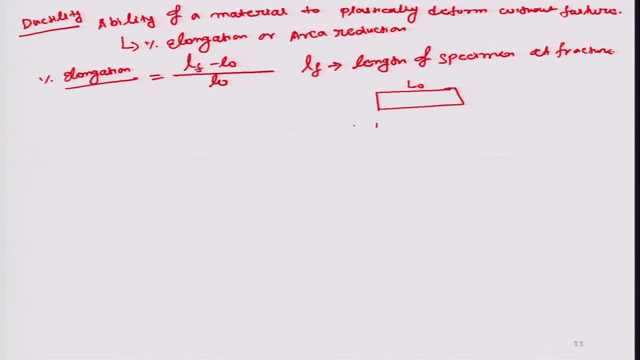 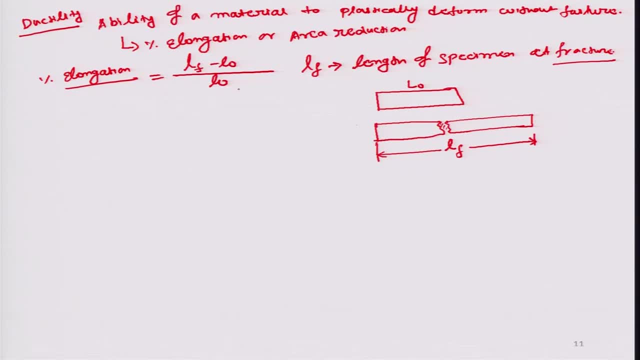 So from here this formula, you can calculate the elong percentage elongation. So from here this formula, you can calculate the elongation of that specimen. Another is area reduction. Again, this is initial cross-sectional area minus cross-sectional of specimen after fracture divided by original cross-sectional area. 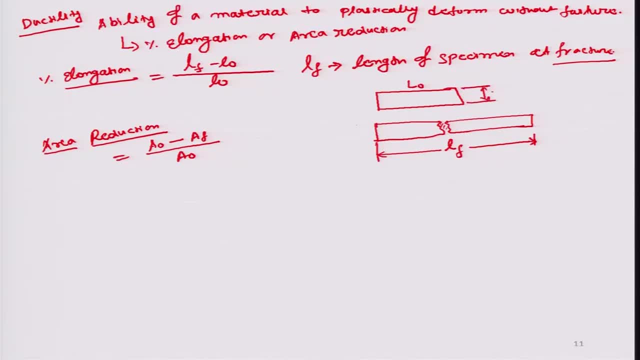 So first suppose that cross-sectional area was A naught Na inside A0 plus nota theta, and now cross sectional area is A f. So after measuring the cross sectional area of the actual cross sectional area, after fracture of that specimen, you can calculate area reduction. 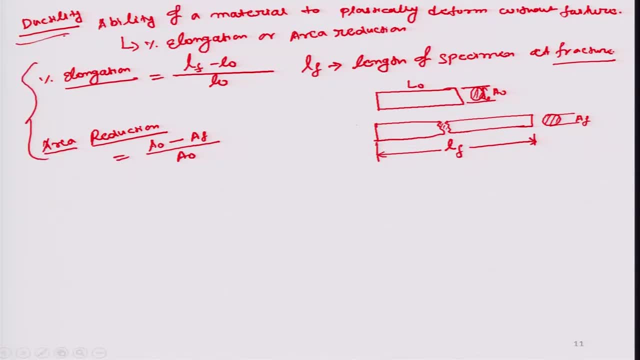 So these both terms defines the ductility of any material. Now, other property is hardness of the material. hardness, it is the resistance of material against abrasion or indentation. Hard rock, weld and Brinell test are used for hardness testing. now the toughness. 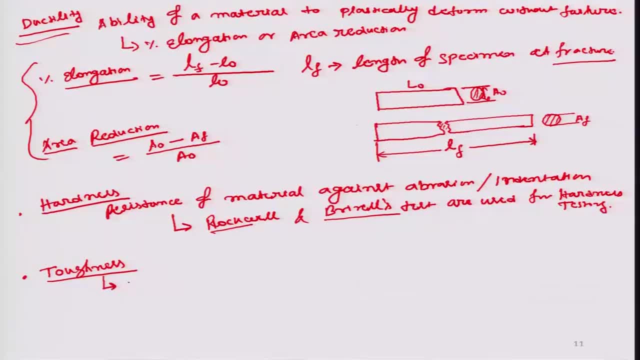 It measures the resistance of a material to the propagation of a crack. 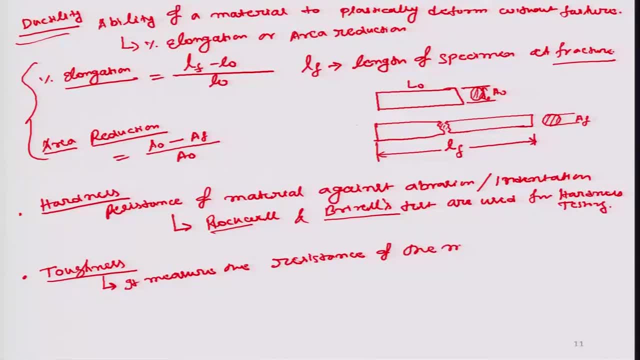 Which are very important during the consideration of selection of material. 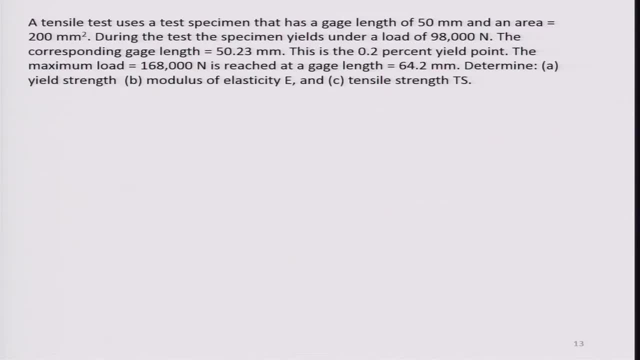 We will do some problem solving example Here. you can see that what problem statement is that a tensile test uses a test specimen that has a gauge length of 50 mm and an area of 20 mm square- that is the cross sectional area During the test, the specimen. 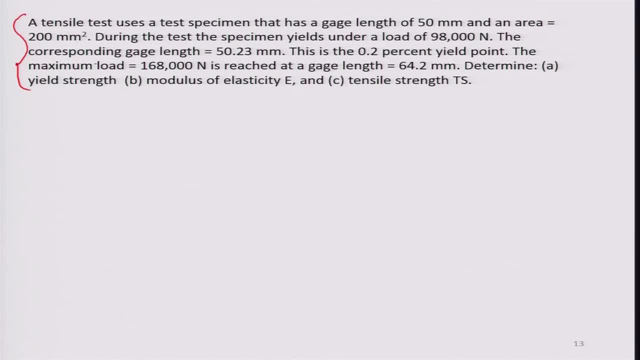 yields under a load of 98000 Newton. the corresponding gauge length is equal to 50.23 mm. this is the 0.2 percent yield point. The maximum load is 168000 Newton. that is the reached at gauge length of 64.2 mm. So determine yield strength, modulus of elasticity and tensile strength. 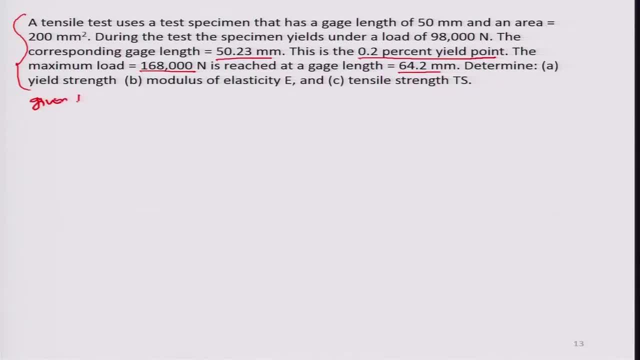 So what are the things given? Given that gauge length of 50 mm L naught is equal to 50 mm A naught is equal to 200 mm square Yield strength of the specimen is equal to. Y is equal to means specimen yields under a load of 98000 Newton. So if you want to, 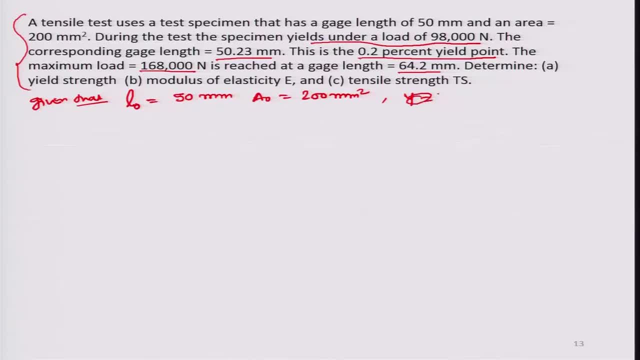 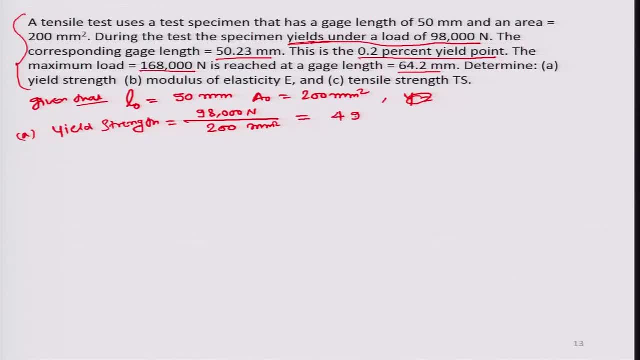 that will be 490 mega Pascal, or is equal to Newton. either you can write Newton per mm, equal to newton, either you can write newton per mm square. ok now modulus of elasticity. modulus of elasticity, we can calculate by Hooke's law what it states: yield strength. 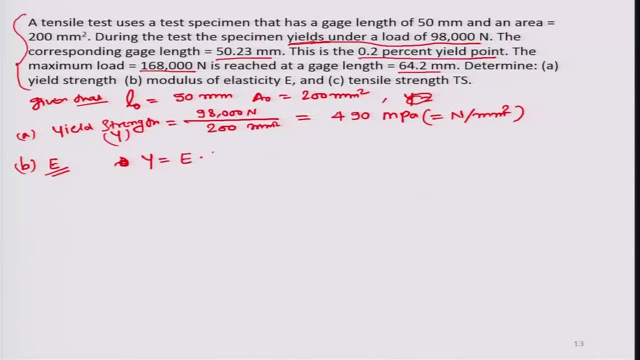 y is equal to young's modulus into strength, this one. so e is equal to y by e. so what is the strength? so first we will see: original gauge length was 50 mm. corresponding gauge length is 50.23 mm and there is a 0.2 percent yield point. earlier I had discussed that the 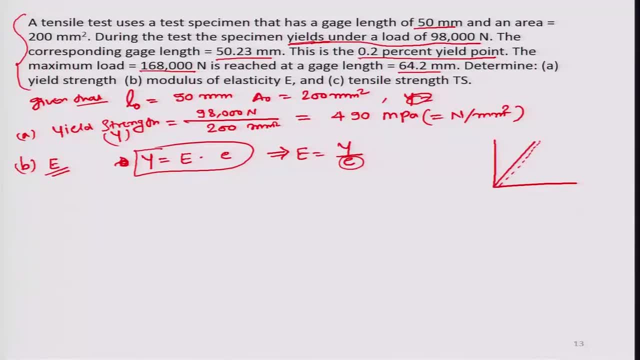 for yield point. there is a one parallel line is calculated. so 0.2 percent, that is the yield point, 0.2 percent. ok, so if you calculate the strength, change in length will be 50.23 minus 50 and original length. so in this case, original, what? 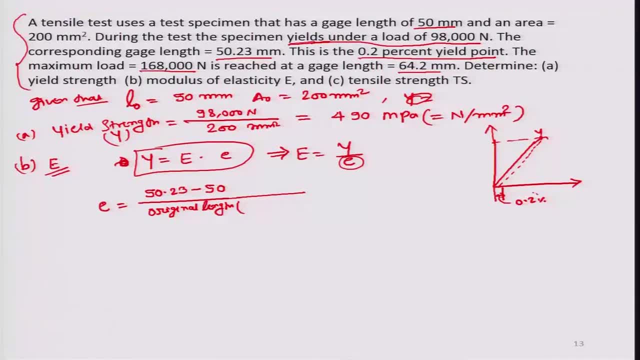 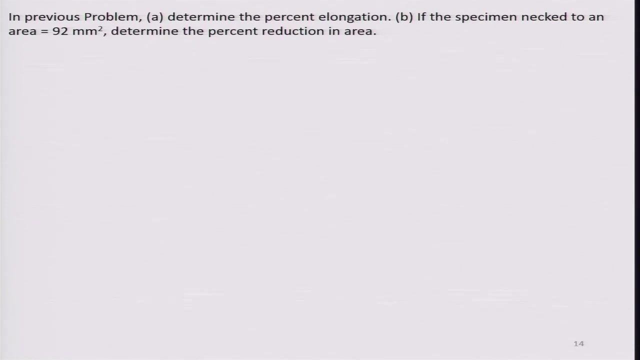 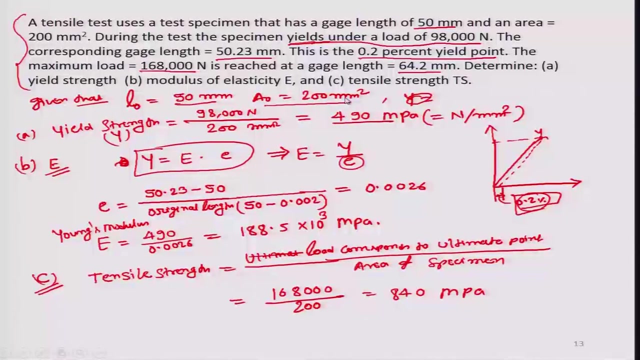 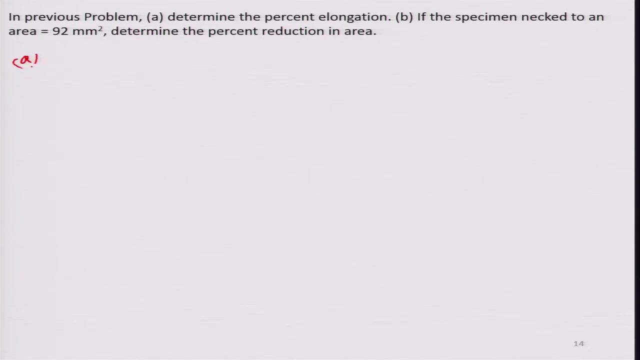 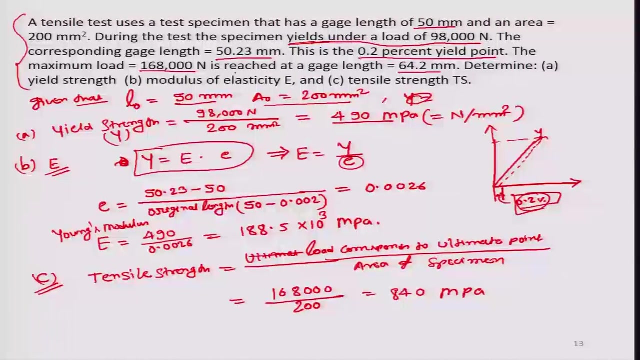 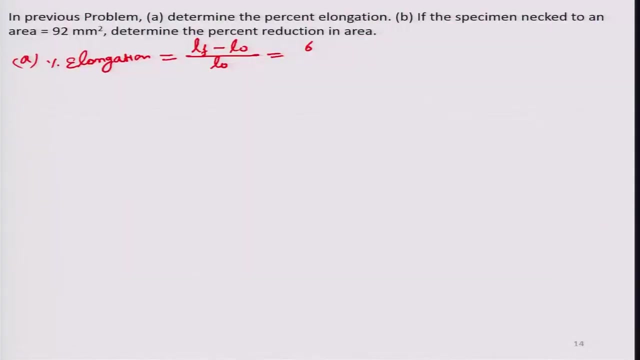 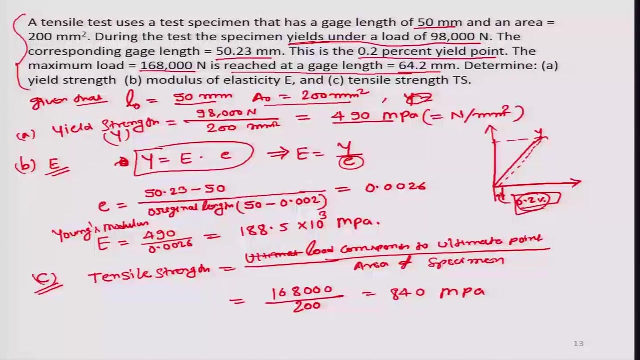 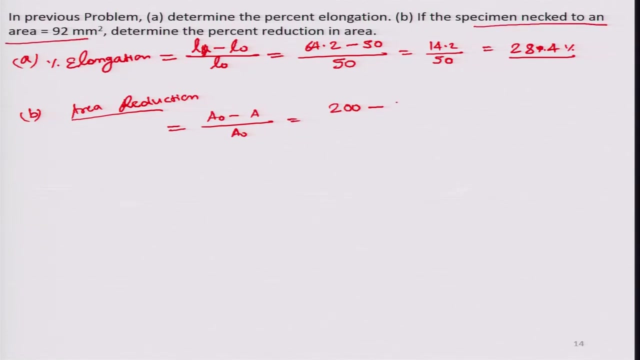 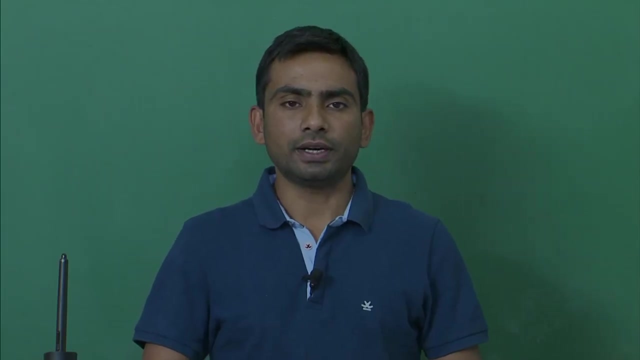 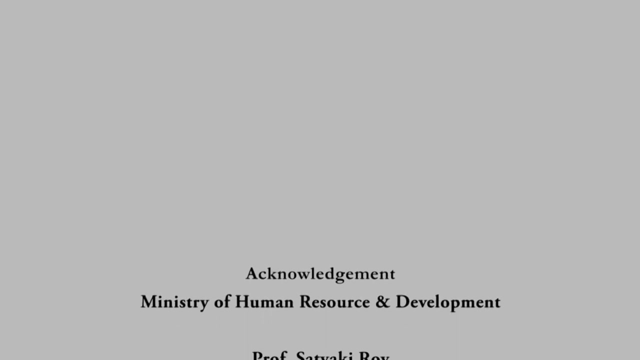 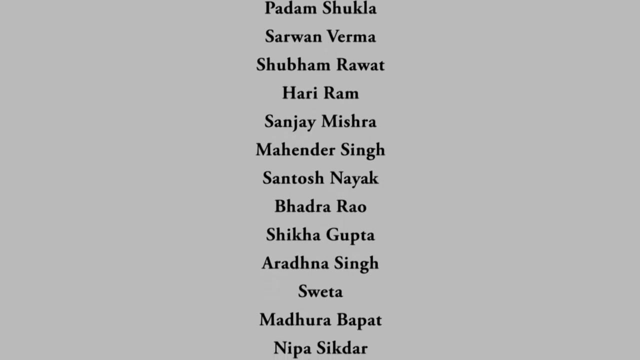 will be original length. actually we omitted this. that amount of strength 0 for, we consider taken. we take 0.2 percent strength for 0.2 percent.